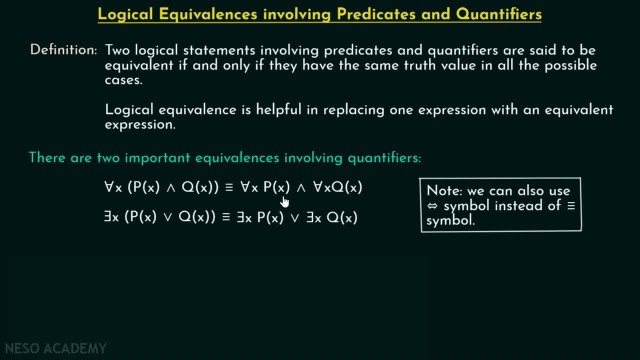 When I say for all x, px and qx is equivalent to for all x, px and for all x, qx, what do I mean is that for all x, px and qx implies for all x, px and for all x, qx. 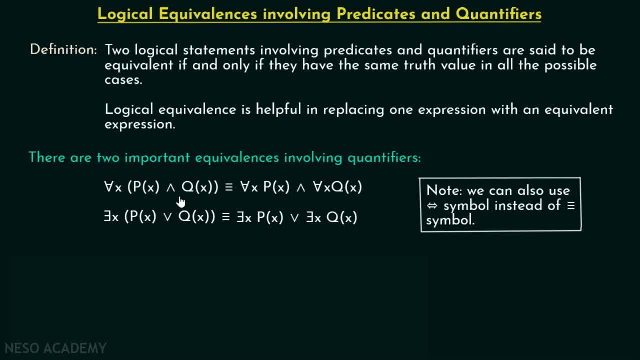 Also, for all x, px and for all x, qx implies for all x, px and qx. 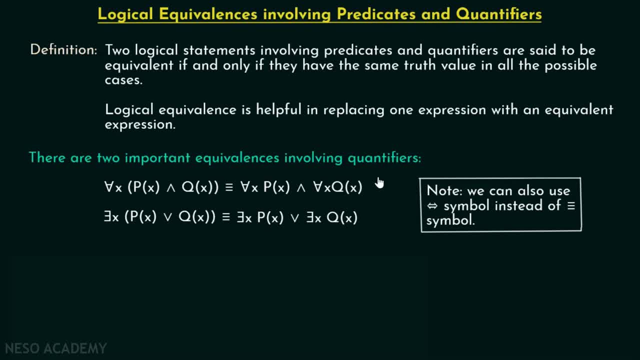 This is the meaning of equivalence. You should think of this that this is the combination of forward implication as well as backward implication. 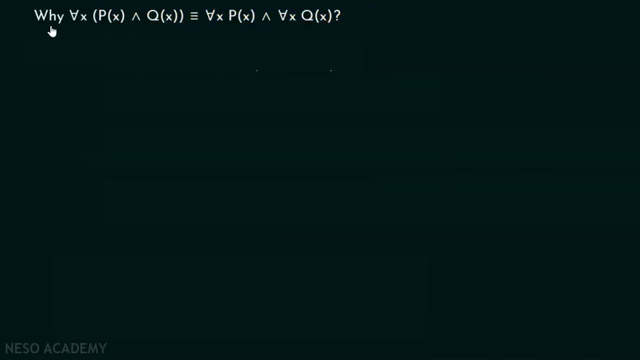 So, equivalence means the same thing. Now, I would like to ask this question that 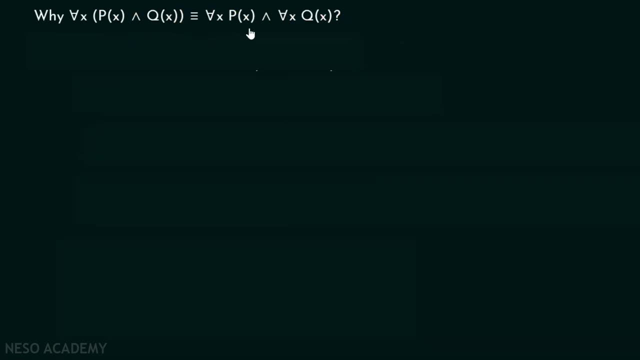 why for all x, px and qx is equivalent to for all x, px and for all x, qx. 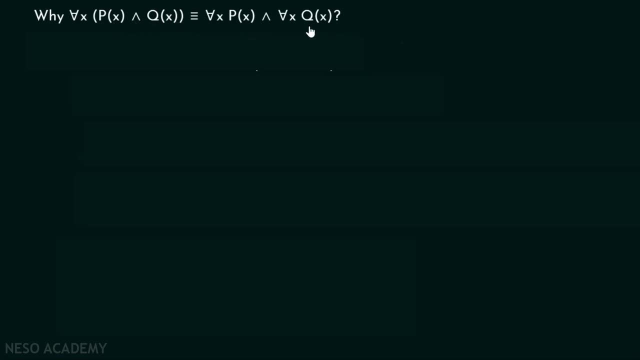 Why is that so? Why these two statements are equivalent? 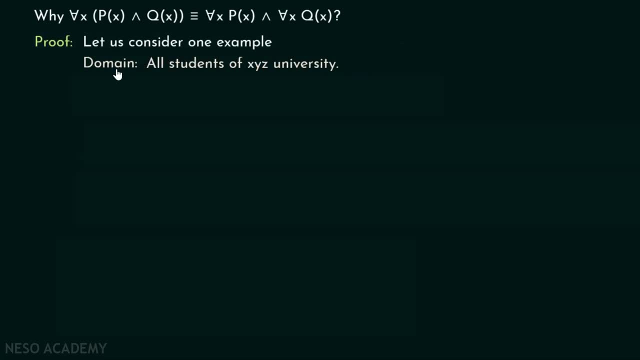 Let us try to prove this with the help of an example. Here we will consider one domain that is all students of x, y, z university. 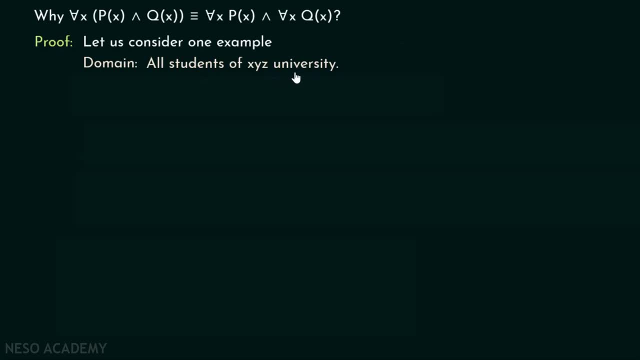 I have considered this domain of all students of some x, y, z university. And I am also considering the predicate px which denotes x has studied discrete mathematics and qx which denotes x has scored more than 60% marks in exam. Now, here comes the statement that is for all x, px and qx. 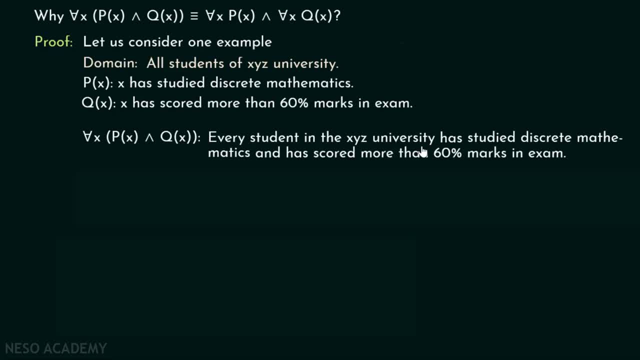 This statement can be replaced by this statement that is every student in the x, y, z university has studied discrete mathematics and has scored more than 60% marks in exam. For all x, px and qx. 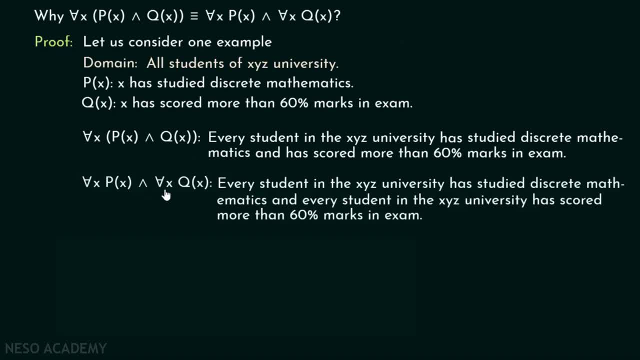 Similarly, we can also write this statement that is for all x, px and for all x, qx in English as every student in the x, y, z university 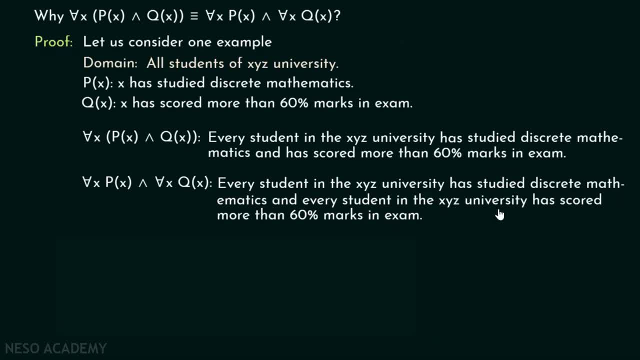 has studied discrete mathematics and every student in the x, y, z university has scored more than 60% marks in exam. So, this is the meaning of this particular statement. 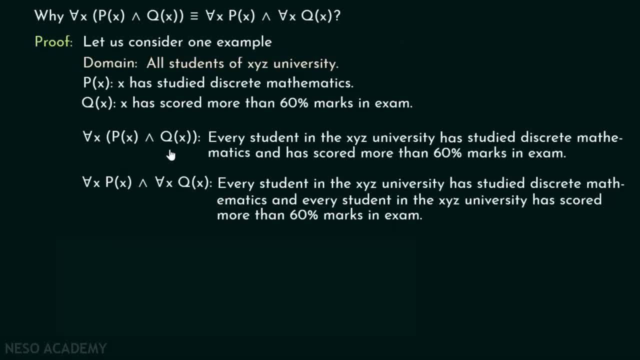 Now, why these statements are equivalent? In order to prove why they are equivalent, we will first prove that for all x, px and qx implies for all x, px and for all x, qx. Then we will prove for all x, px and for all x, qx implies for all x, px and qx. 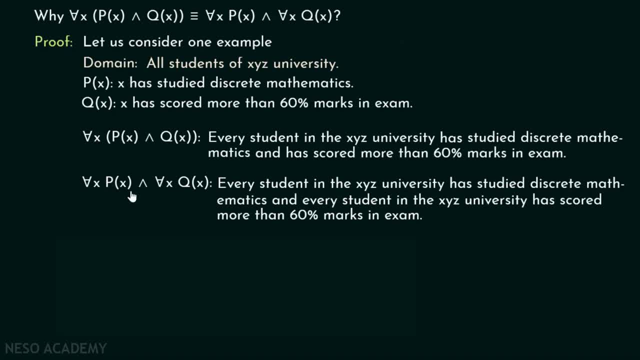 Now, what is the meaning of for all x, px and qx implies for all x, px and for all x, qx? It means that when this particular statement is true, then this cannot be false. If this becomes false, then it means that implication becomes false, right? So, let us suppose that for all x, px and qx is true and then we will prove that for all x, px and for all x, qx will definitely be true. 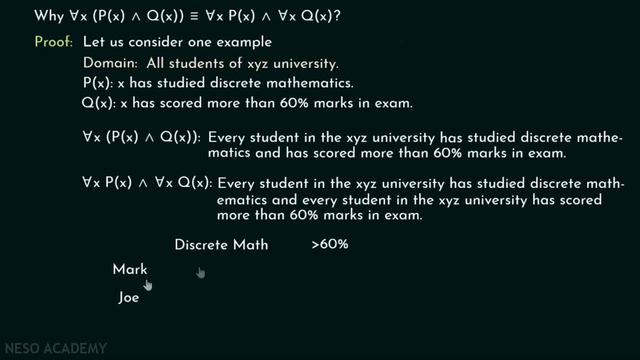 For this purpose, I have written Mark and Joe, the names. 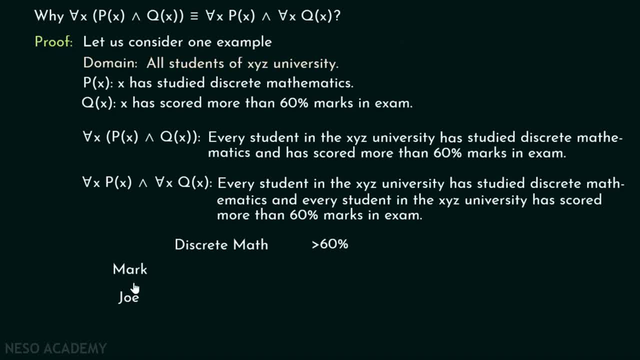 I am considering that the XYZ university has these two students only. This is my hypothetical university. 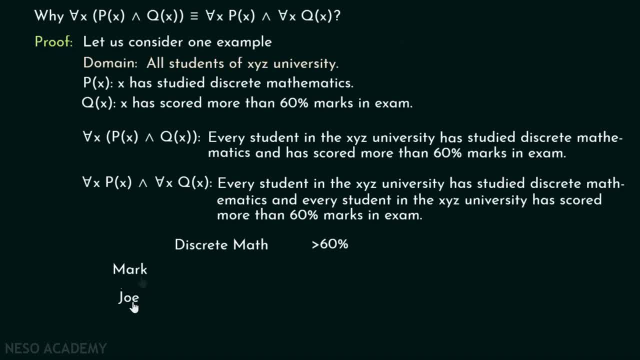 In this university, we have only these two students, Mark and Joe. 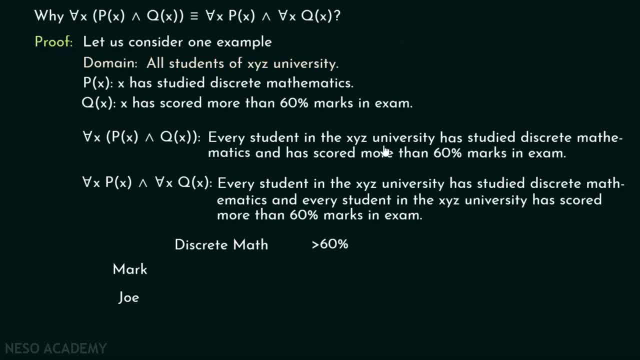 Now, I am considering this statement, that is every student in the XYZ university has studied discrete mathematics and has scored more than 60% marks in the exam. 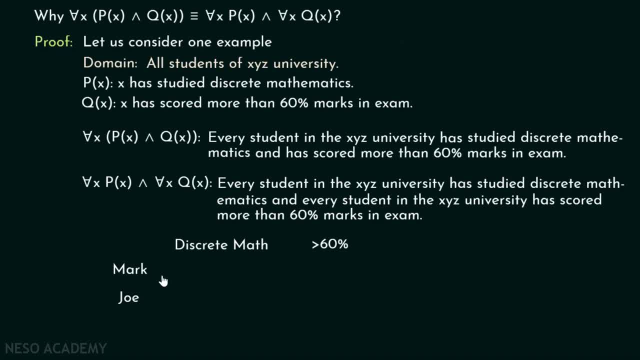 We know that Mark and Joe are the students of this university and they are the only students of this university. 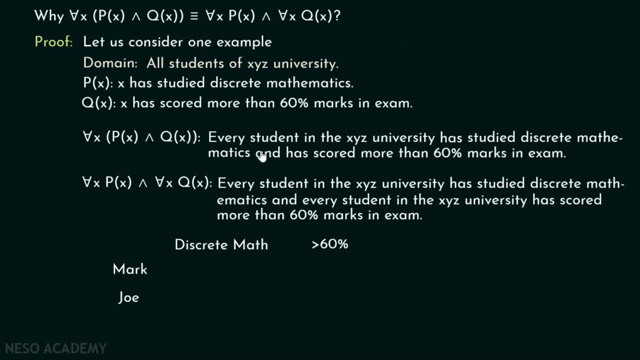 Now, if I am saying that this statement is true, then this means that Mark has studied discrete mathematics 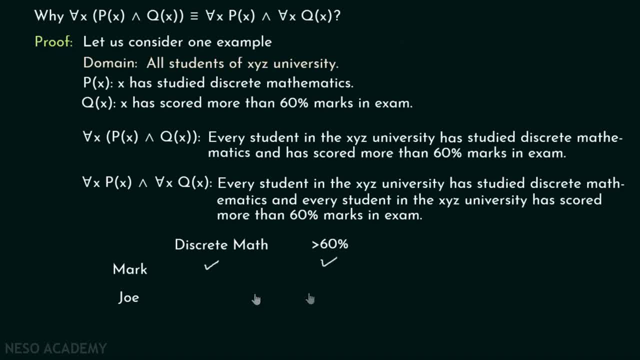 also, he has scored more than 60% marks. 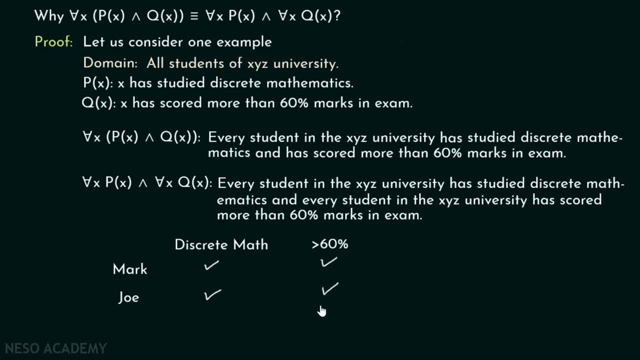 And Joe has also studied discrete mathematics and he has also scored more than 60% marks. 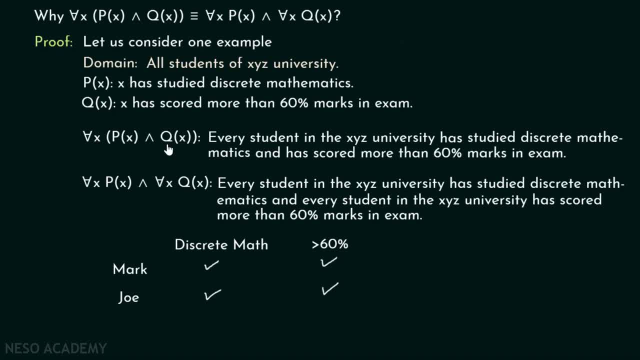 Right? This is what the statement is saying. Now, as this statement is true, let us find out whether this statement is true or not. Every student 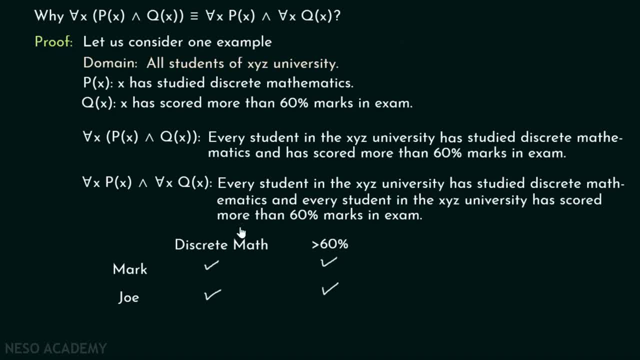 in the XYZ university has studied discrete mathematics. Is it true? Yes, of course. You can see over here that every student has studied discrete mathematics. 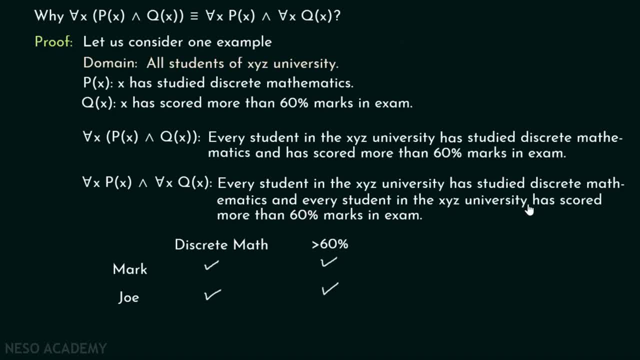 And every student in the XYZ university has scored more than 60% marks in the exam. 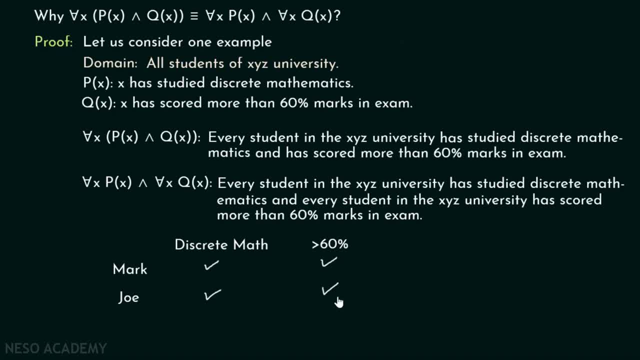 Is this true? Yes, of course. You can see over here that this is also true. So, we can say that, for all x px and qx, this implies for all x px and for all x qx. This is true. For all x px and qx implies for all x px and for all x qx is true. When this is true, this can never be false. 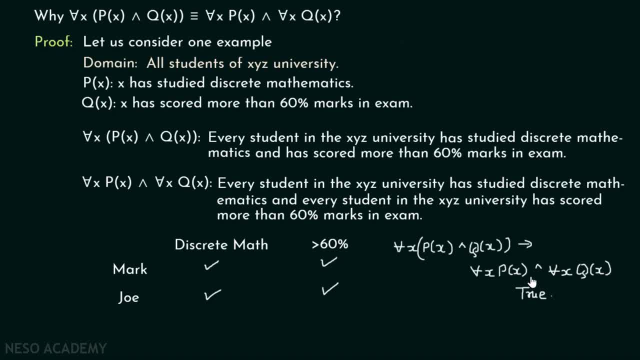 That is why this implication is satisfied. Now, let us consider the backward implication, that is, for all x px and for all x qx implies for all x px and qx. 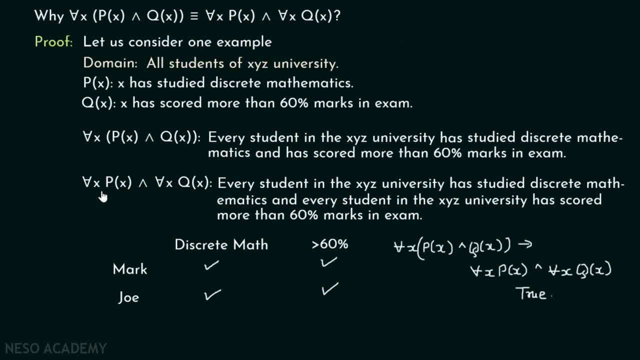 Let us see whether this is true or not. For this purpose, we have to consider for all x px and for all x qx is true and then we will prove for all x px and qx is true. Here you can see that 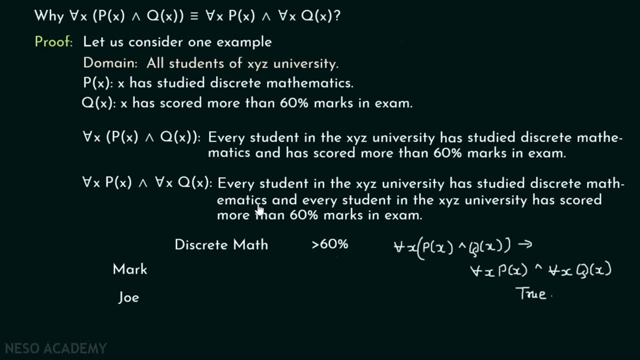 every student in the XYZ university has studied discrete mathematics. 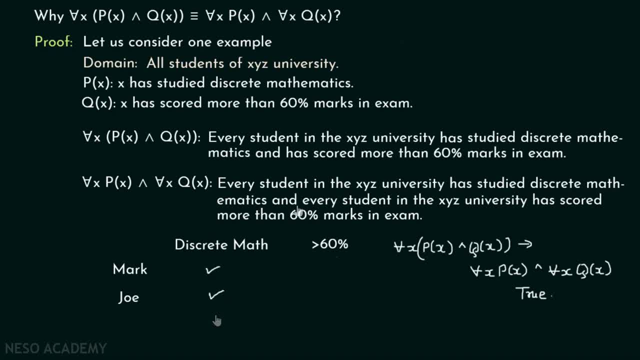 So, this means that Mark and Joe has studied discrete mathematics. 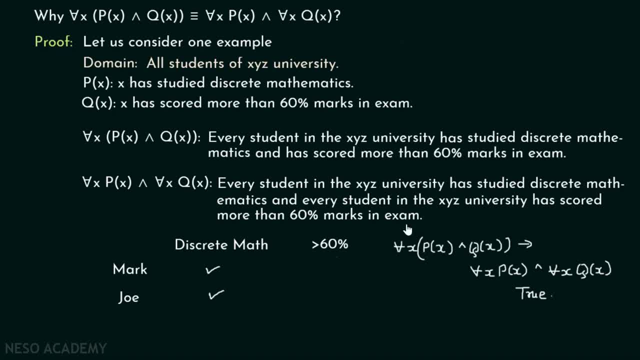 And every student in the XYZ university has scored more than 60% marks in exam. 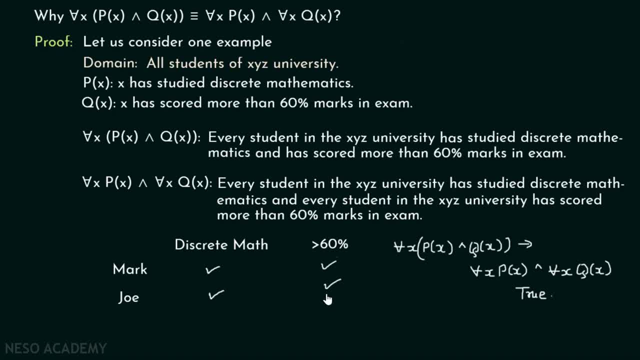 So, this means that this one is also satisfying. Then, we can clearly say that for all x px and qx will definitely be true. 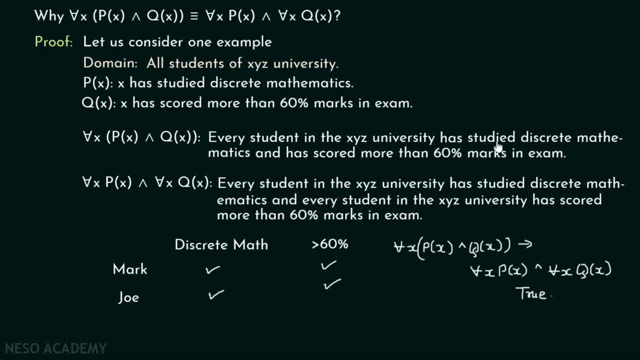 Because here we are saying every student in the XYZ university has studied discrete mathematics and has scored more than 60% marks in exam. You can see over here that 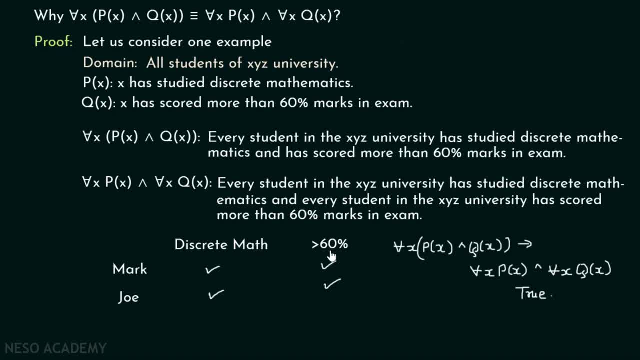 every student has studied discrete mathematics and has scored more than 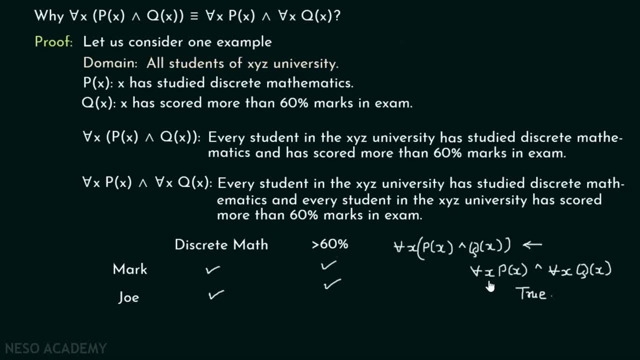 60% marks. So, we can clearly say that for all x px and for all x qx, when this is true, then this will definitely be true. Hence, this is also satisfied. 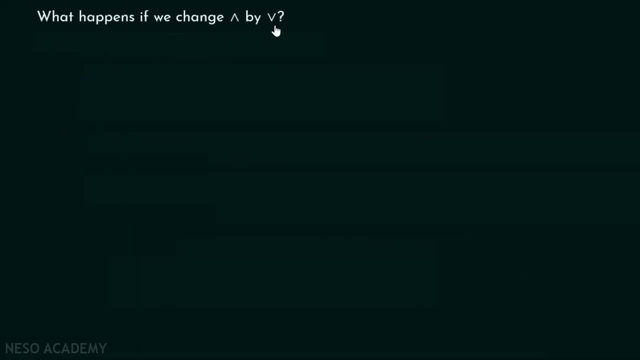 Now, let us consider what happens if we change AND by OR. That means something like this. 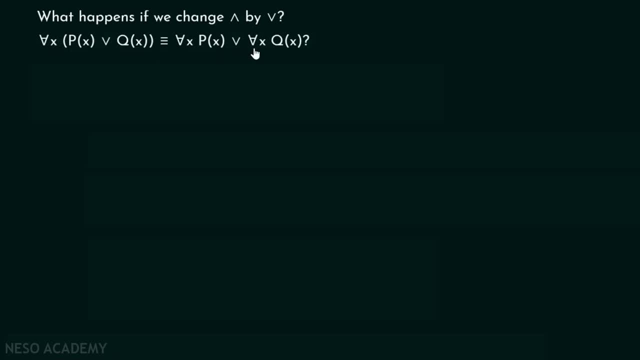 For all x px or qx is equivalent to for all x px or for all x qx. Are they equivalent? Let's try to find out. 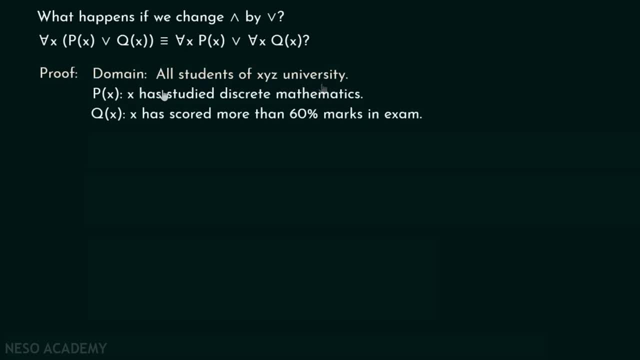 I am considering the same domain that is all students of XYZ university. I am considering this predicate px as x has studied discrete mathematics and qx as x has scored more than 60% marks in exam. Then, for all x px or qx will be every student in the XYZ university has studied discrete mathematics or has scored more than 60% marks in exam. 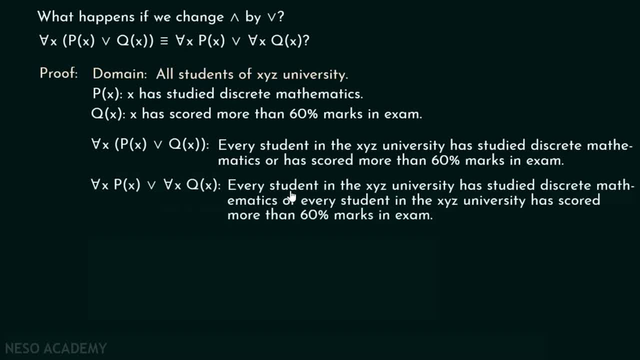 This is what this statement means. And here this statement means every student in the XYZ university has studied discrete mathematics or every student in the XYZ university has scored more than 60% marks in exam. 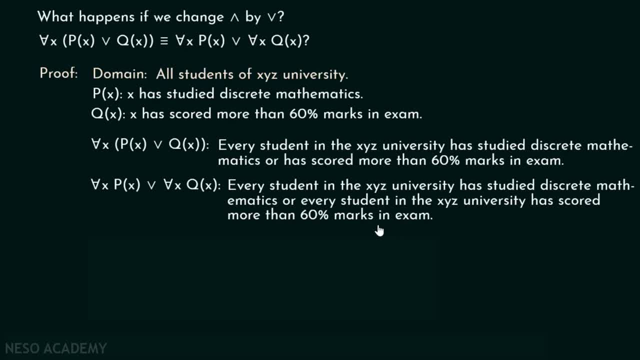 In order to prove this, again we will consider the same case. That is, we will consider the first forward implication that is for all x px or qx implies for all x px or for all x qx. Let us consider 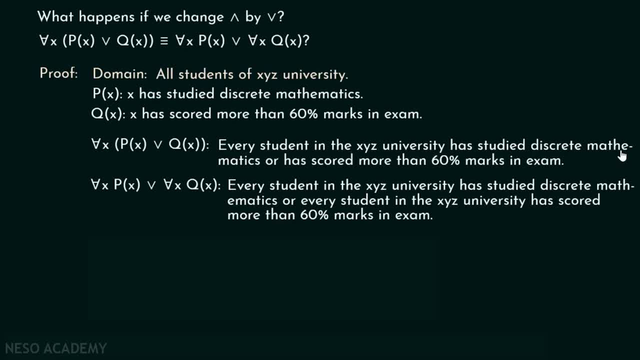 this statement is true. That is, every student in the XYZ university has studied discrete mathematics or has scored 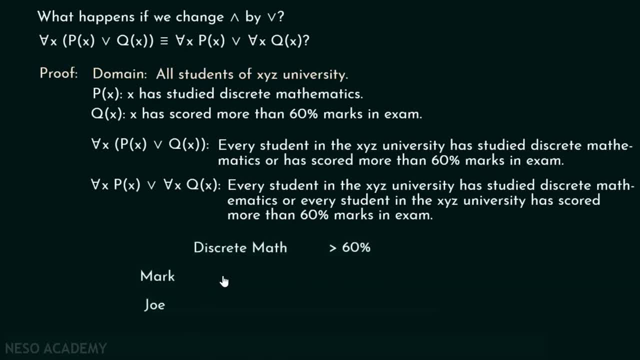 more than 60% marks in exam. Let us suppose that Mark has studied discrete mathematics but he has not secured more than 60% marks. And I am also considering that Joe has not studied discrete mathematics but he has scored greater than 60% marks. So, this statement is satisfied. Isn't that so? Now, let us consider this statement. 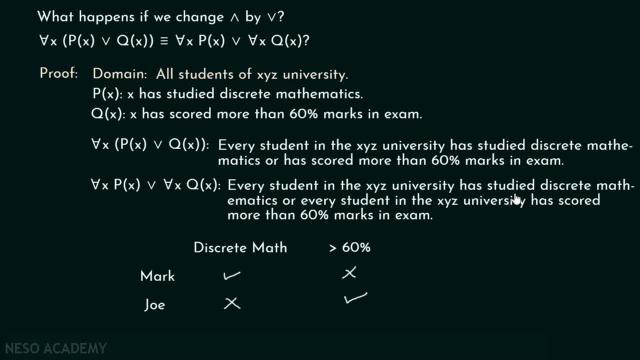 For all x px or for all x qx. That is, every student in the XYZ university has studied discrete mathematics. Is it true? 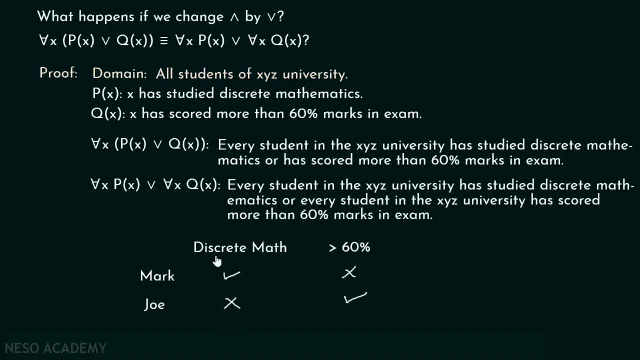 No. Not every student has studied discrete mathematics. We can see 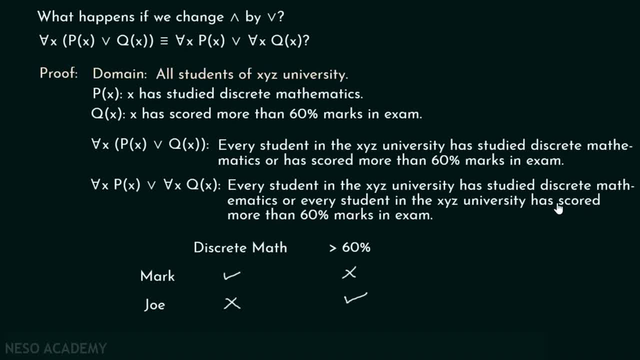 over here. Or, every student in XYZ university has 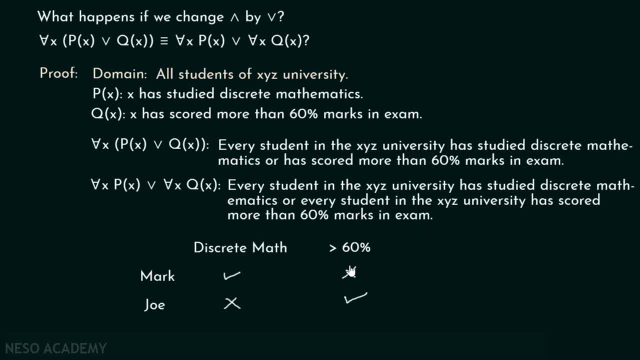 scored more than 60% marks in exam. Again, it's a big no. You can see over here, not every student has scored more than 60% marks. 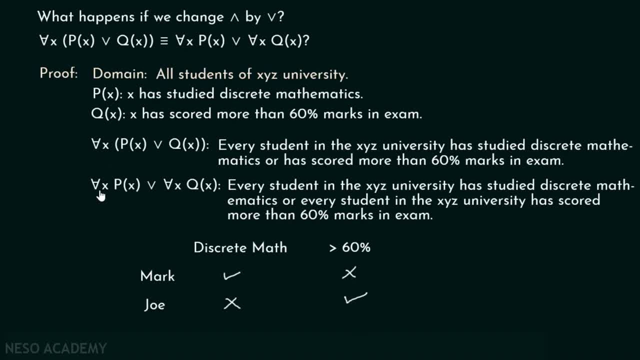 So, what is the conclusion? When this is true, this becomes false. Right? So, this means that forward implication is not satisfied. That is, for all x px or qx implies for all x px or for all x qx is false. As this is false, then equivalence cannot be true. 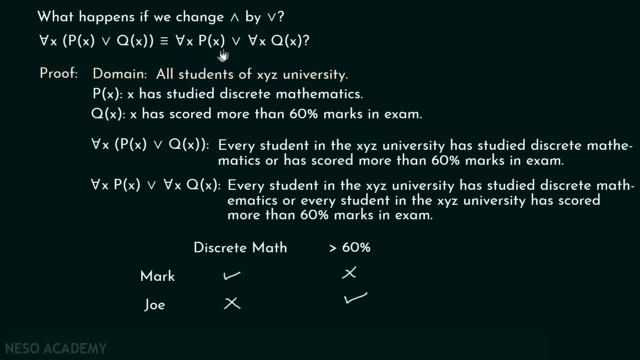 These statements are not equivalent. Isn't that so? If any 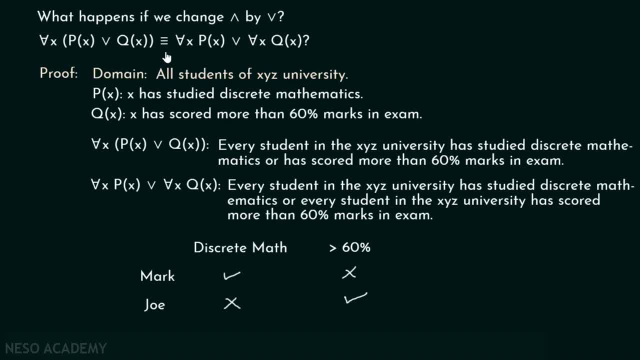 of the implication is not satisfied, then this means that equivalence is not satisfied. So, what is the conclusion? 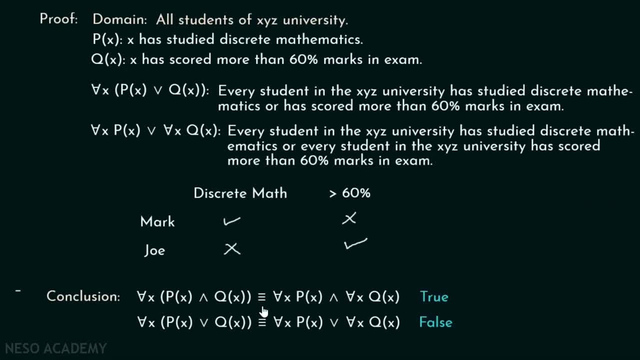 Conclusion is that for all x px and qx is equivalent to for all x px and for all x qx, but for all x 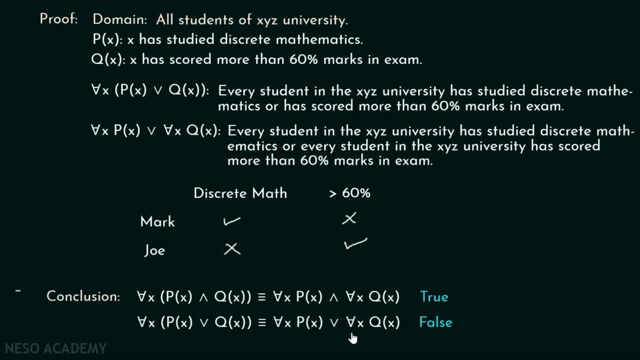 px or qx is not equivalent to for all x px or for all 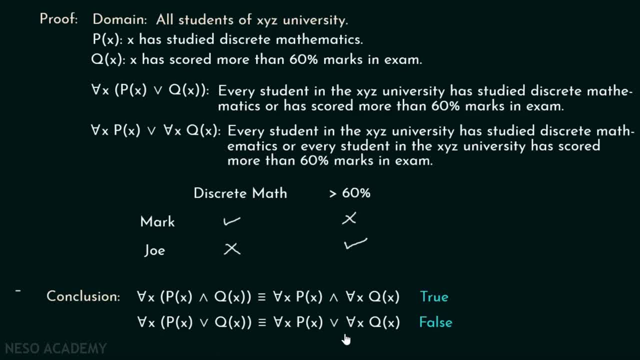 that these two statements are equivalent, but these two statements are not. 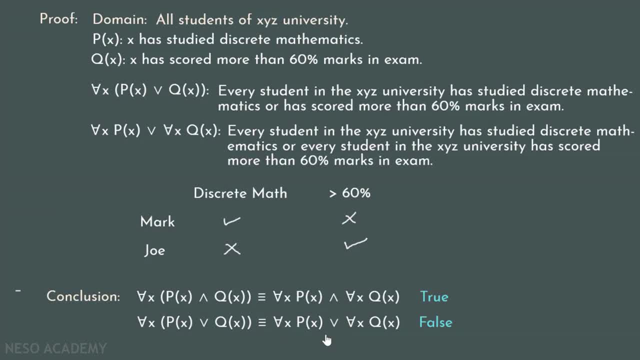 You can't replace AND by OR and say that they are equivalent.